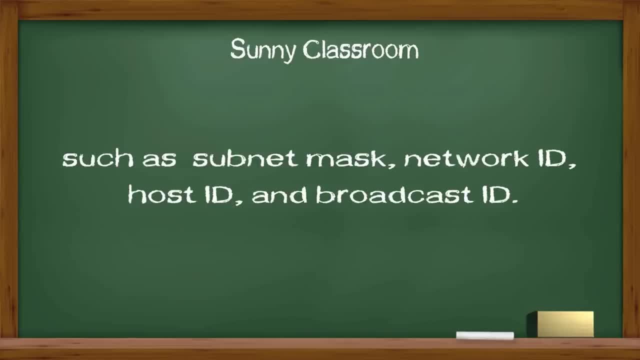 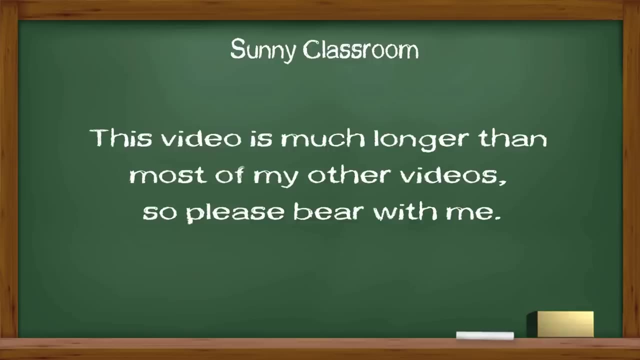 basic knowledge, such as subnet mask, network ID, host ID and broadcast ID. I put several information on this. Let's take a look now. Here you see the system. I am using network video links below just in case you need them. One more point: this video is much. 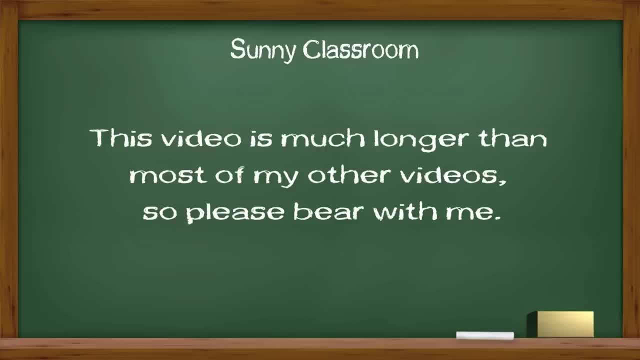 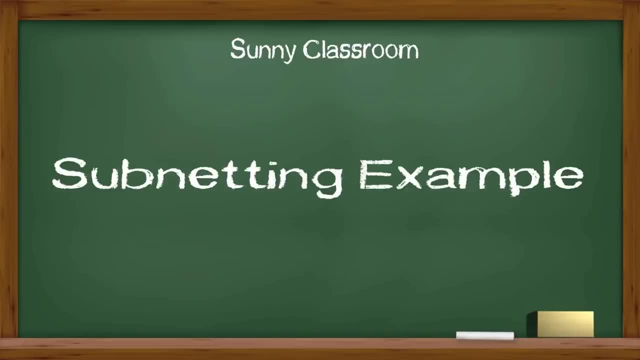 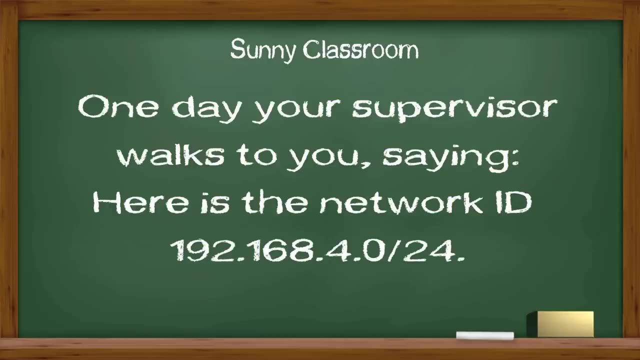 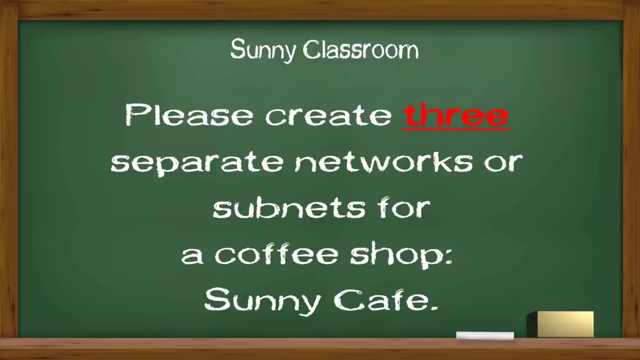 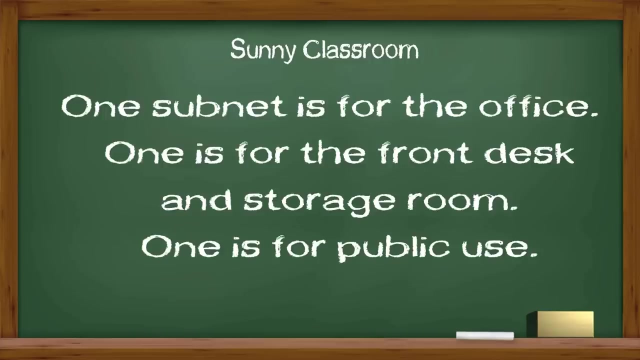 longer than most of my other videos, so please bear with me. Let's take a look at one example. One day, your supervisor walks to you saying: here is the network ID. Please create three separate networks for a coffee shop: one is for the office, one is for the front desk and storage room. 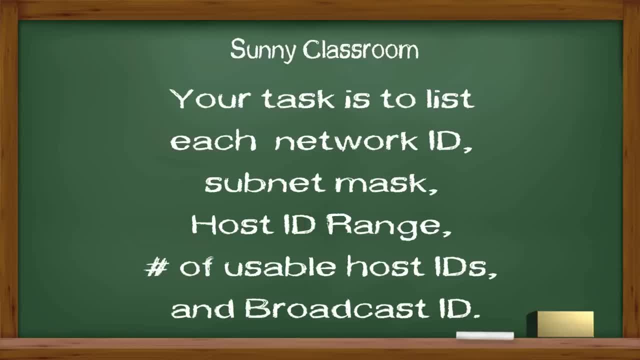 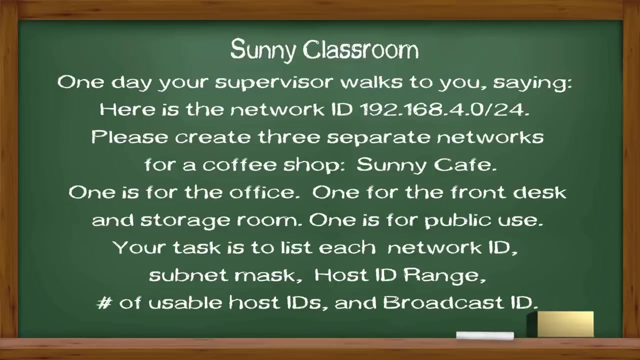 and one is for public use. Your task is to list each subnetwork ID, subnet mask, host ID range, the number of user ID and broadcast ID. I put this example below this video so that you can copy it to your document for your reference as we discuss. 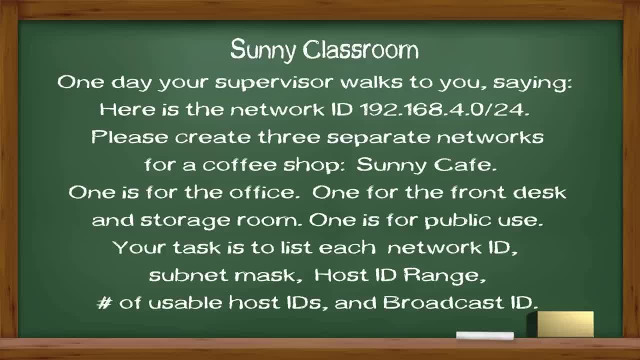 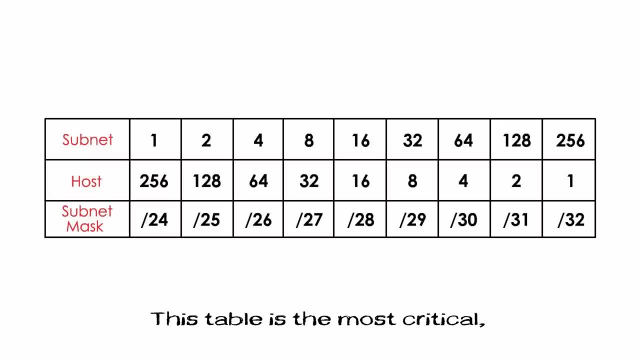 the process of subnetting First is: first let's build a table. This table contains four subnetwork ID. the main one for this video is the subnetwork ID This. This table is the most critical because once we build it we can easily solve most subnetting. 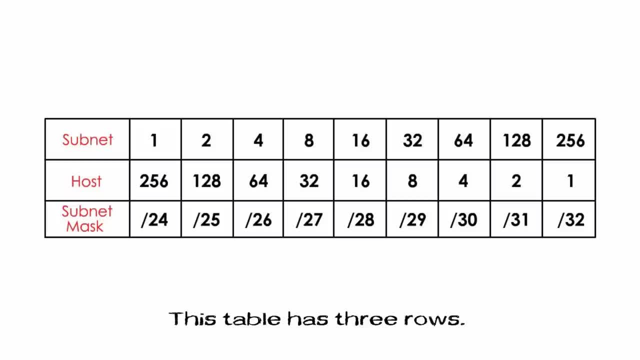 questions And this table has three rows. The first row is subnet with nine numbers. We start with 1, then 2,, 4,, 8,, 16,, 32,, 64,, 128, and 256.. The pattern is: each number is a double of its previous number. 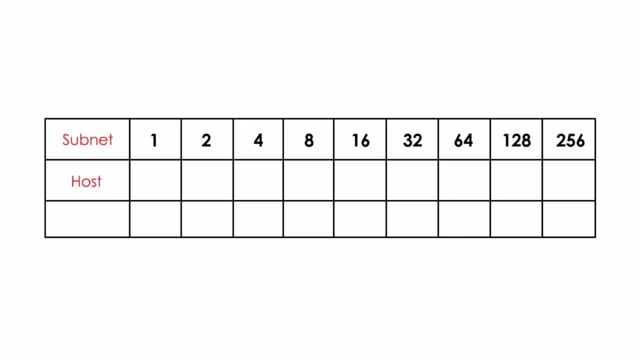 The second row is host. This row tells the number of total host IDs for each new subnet. Start with 256, then 128,, 64,, 32,, 16,, 8,, 4,, 2, and 1.. 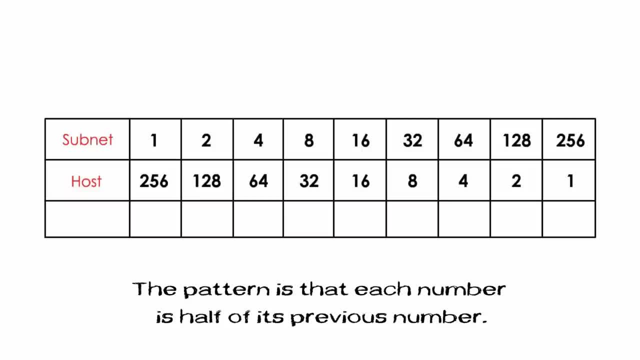 The pattern is: each number is half of its previous number or the second row is the reverse order of the first row. You see, everyone can handle this right. The third row is the subnet mask. We use shorthand format starting with 24,, 25,, 26,, 27,, 28,, 29,, 30,, 31,, 32.. 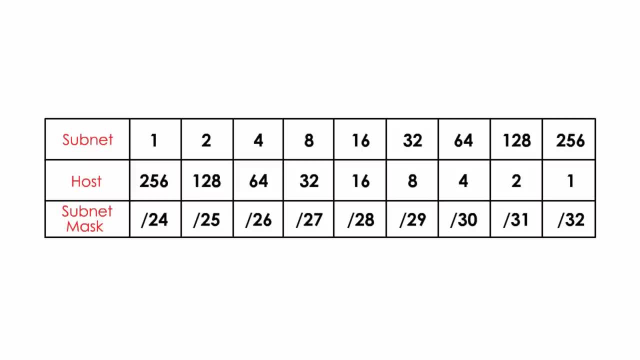 Well, we are done. I call this table sunny subnetting table or simply sunny table, because it's a simple sunny. We write a number for table for subnetting and subnetting a subnet. Now we use sunny table to solve the subnetting example mentioned above. 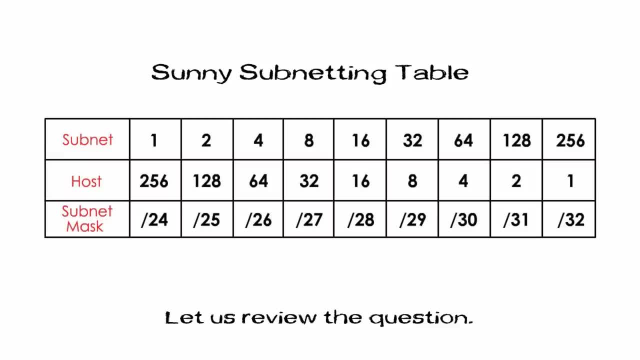 Let's go back to the question. You are given a network ID, 192.168.4.0/.24.. Is subnet mask. You are required to get three subnets right. Ok, good, three subnets. Three is the key, key word. 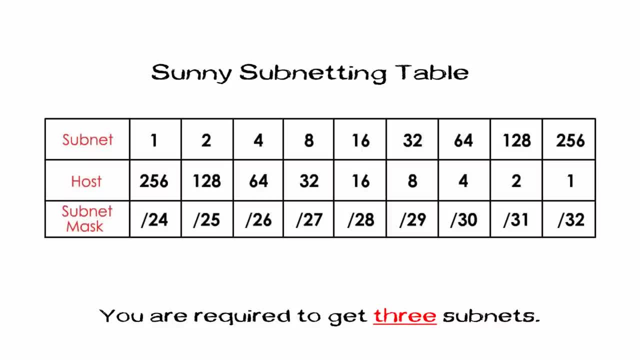 Now look at the sunny table and try to find the three subnets in the first or in the top row. Of course there's no exact three subnets, but four subnets are suitable because we can get four subnets and choose any three subnets. 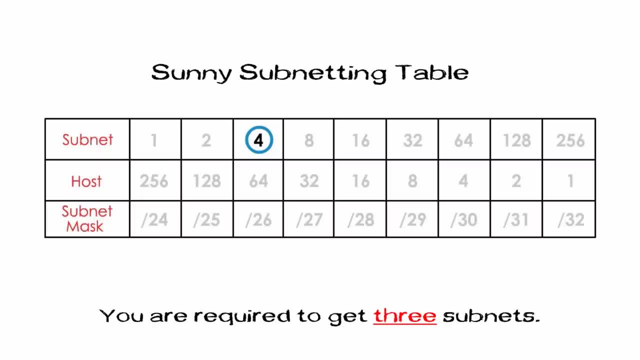 for sunny cafe. So we choose four, subnets, four. Let me circle the whole column, ignoring all other columns, because we only use these three numbers and we can get all our answers just from this column, or these three numbers: Four, sixty-four and slash twenty-six. 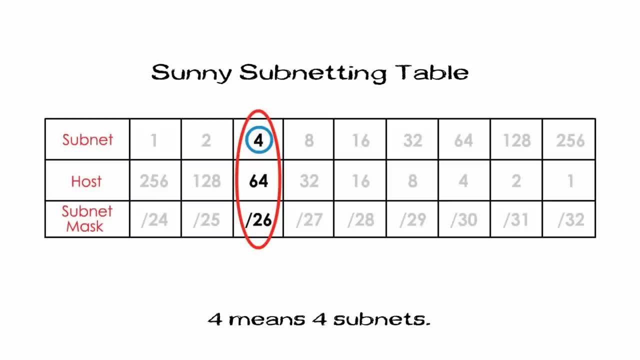 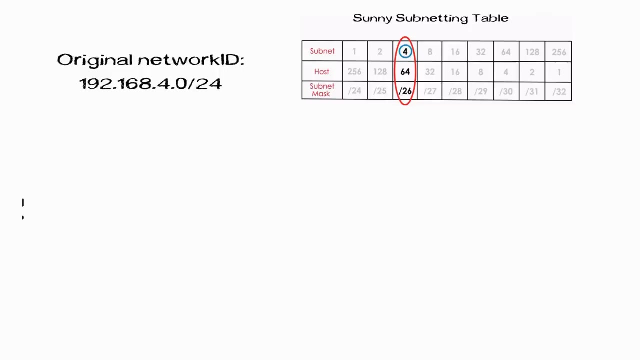 Four means four subnets. Sixty-four means each subnet. each new subnet will have sixty-four total host IDs, including network ID and broadcast ID. Slash twenty-six is the new subnet mask for all these four subnets. Well, let's list all these four subnets'. 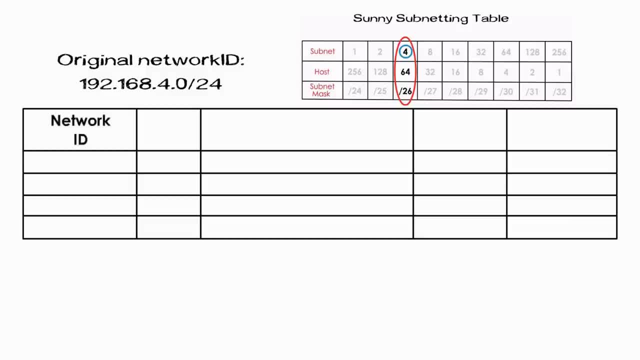 information: Network ID, subnet mask, host ID range, the number of usable host IDs and broadcast ID. Let's find the first network ID. The first network ID is always the original network ID, which is 192.168.4.0.. That's easy, right. 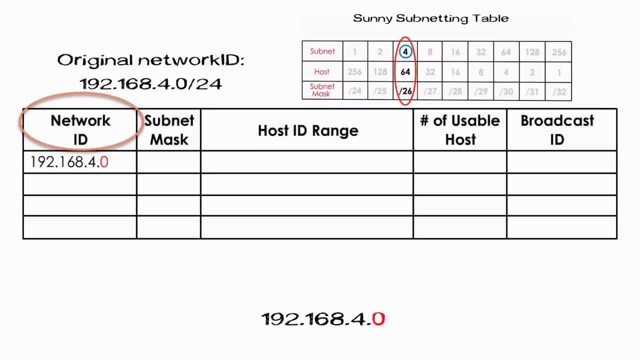 I use red font to emphasize the last number because the first three numbers stay the same across the table, So please just focus on last number in red. We will get next the second network ID by simply adding sixty-four to its previous network ID, Therefore the second. 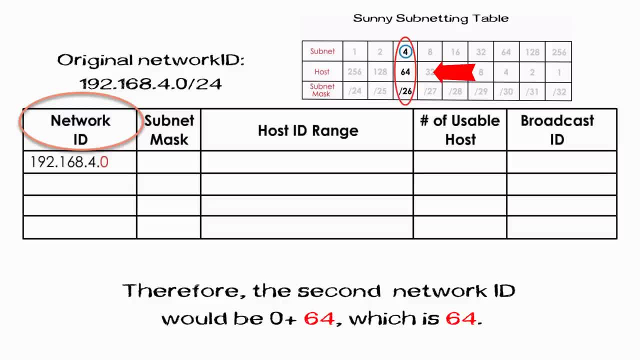 network ID is zero plus sixty-four, which is sixty-four. The third network ID would be sixty-four plus sixty-four, which is one-twenty-eight. The fourth network ID is one-twenty-eight plus sixty-four, which is one-ninety-two. 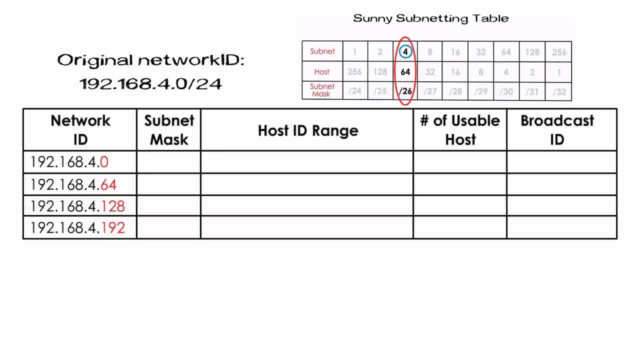 Now subnet mask for each subnet. Well, they are all slash twenty-six. The original subnet mask is slash twenty-four. We are done with the subnet mask column. Now let's list the number of usable host IDs. We can also find the answer from the Sony table. 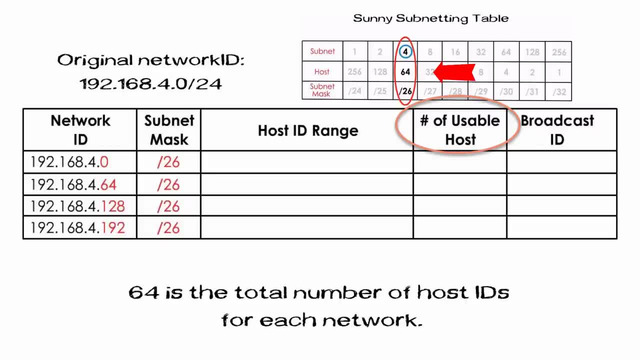 which is sixty-four. Sixty-four is the total number of host IDs for each network or each subnet, But the first host ID is reserved for network ID and the last host ID is reserved for broadcast ID. Thus the number of usable host IDs. 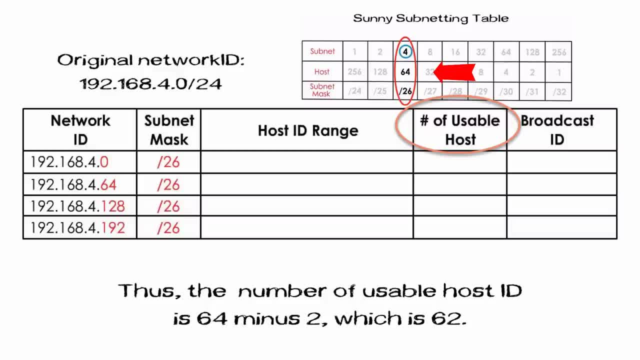 the usable host ID is sixty-four minus two, which is sixty-two. Thus we write down sixty-two for all four subnets. We are done with the fourth column. Now let's look at the broadcast ID for each subnet. Keep in mind, the last host ID is reserved. 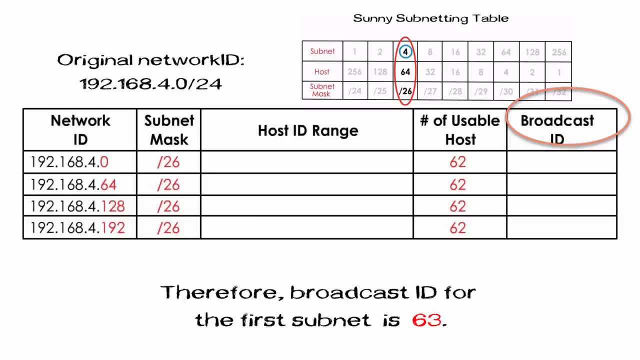 for its broadcast ID. Therefore, broadcast ID for the first subnet is sixty-three And we can tell with the reference to the next network: ID: sixty-four. Next broadcast ID is one-twenty-seven, Next one is one-ninety-one. 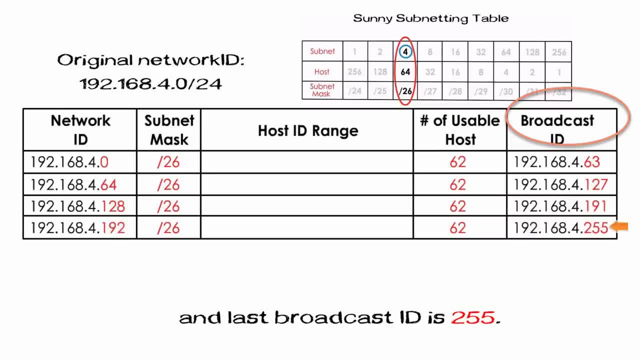 And the last broadcast ID is two-five-five, We can say: the broadcast ID equals next subnet network's ID minus one. We can also do like this: Once you know the first broadcast ID, sixty-three, and then you can simply add sixty-four to get the second broadcast ID. 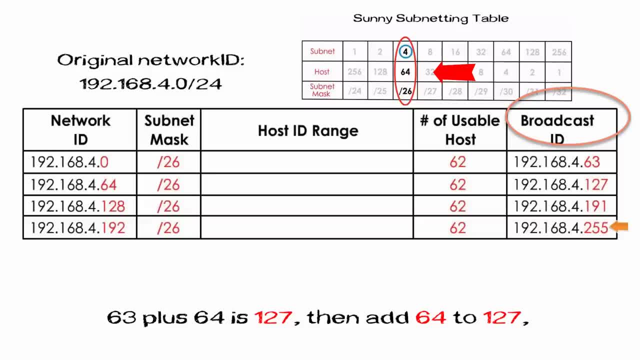 and sixty-three plus sixty-four is one-twenty-seven, And then add sixty-four to one-twenty-seven, which we get the third broadcast ID, one-ninety-one, And then increase by sixty-four again to get the fourth broadcast ID, which is two-five-five. 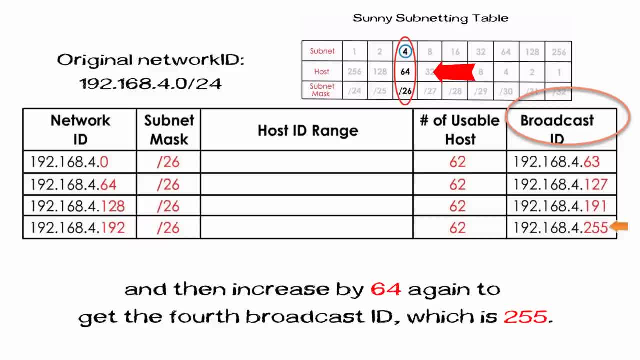 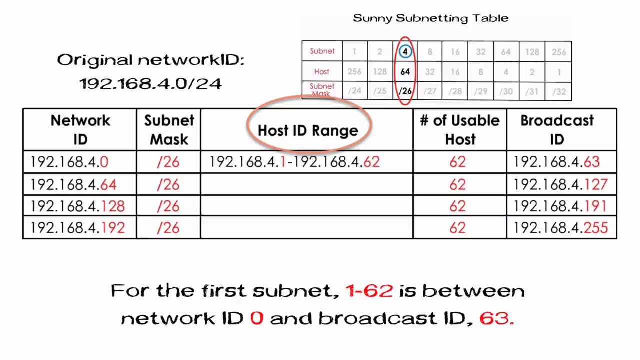 We are almost done. One last column: the host ID range. A subnet host ID range is a subnet host ID range is any IDs between its network ID and broadcast ID For the first subnet. one-two-sixty-two is between network ID zero and broadcast ID. sixty-three 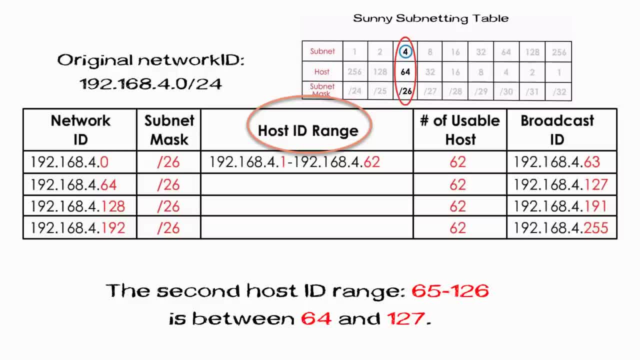 The second host ID range sixty-five to one-twenty-six is between sixty-four and one-twenty-seven. The third host ID range one-twenty-nine to one-ninety is between one-twenty-eight and one-ninety-one. 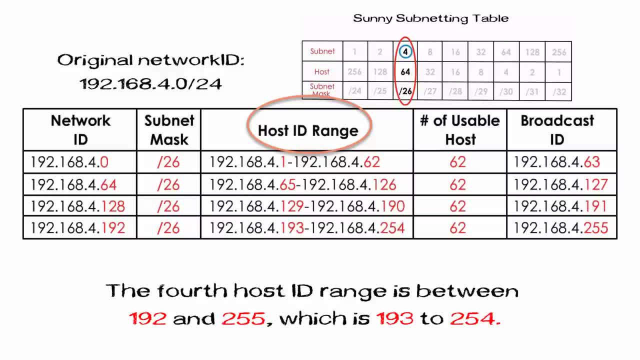 The fourth host ID range is between one-ninety-two and two-five-five, which is one-ninety-three to two-fifty-four. So, to keep simple, we only talk about last number and because the first three numbers state the same, that's all. We get all answers. You can assign any three out of four subnets for Sonic Cafe. One subnet is wasted. of course, That's the downsides of subnetting. No biggie. I want to thank you for following me at this point. 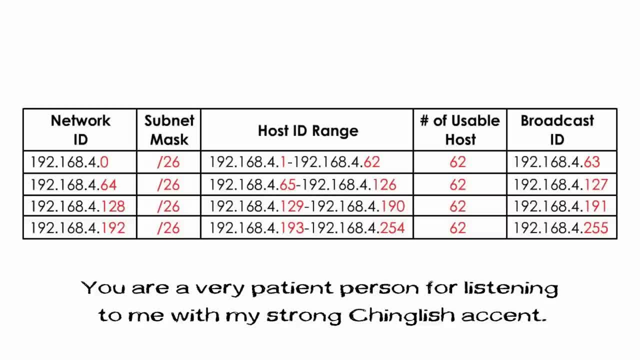 You are a very patient person for listening to me with my strong Chinglish accent, even though the process sounds tedious. But once you get to know how to do it you can solve any similar questions in no time. I put one similar question below for your practice. 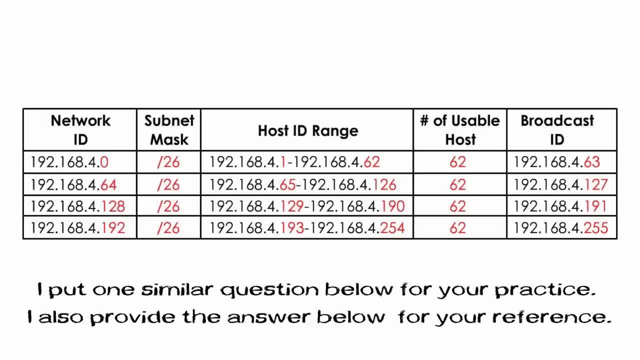 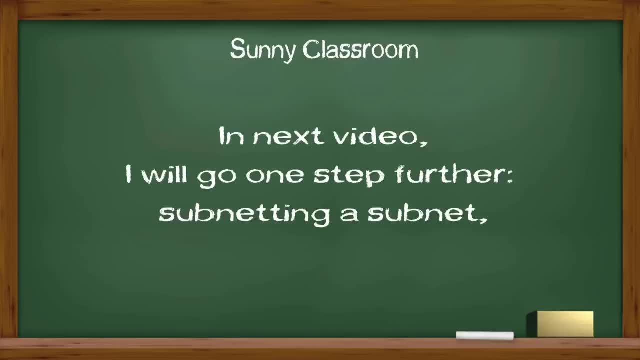 I also provide the answer below for your reference. If you have questions, please feel free to leave your comments or ask me questions. I would be happy to help you. In next video I will go one step further: subnetting a subnet. 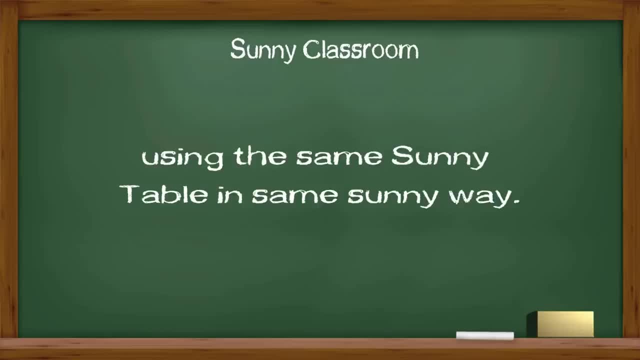 using the same Sonic table in same Sonic way. Please stay tuned. Thank you very much and see you next time. Subtitled by Grethel Trejo.